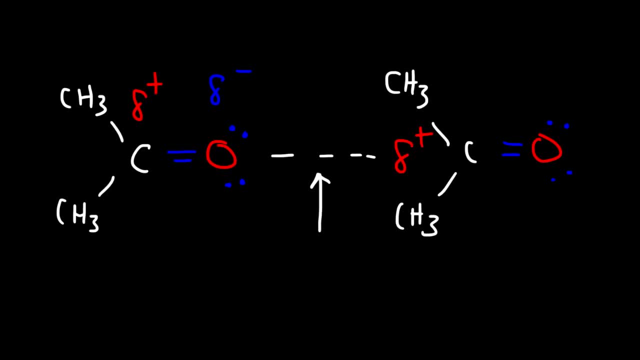 within a molecule. Let's consider another example, And that is carbon monoxide, which looks like this: The carbon bears a partial positive charge and the oxygen bears a partial negative charge. And let's draw another carbon monoxide molecule next to it. 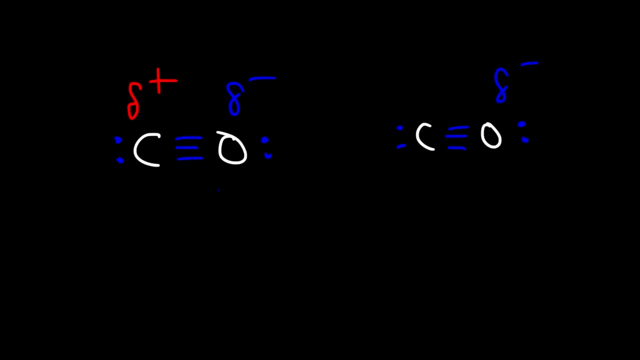 So each of these molecules possess a dipole moment, And so you can call it a dipole, And so the interaction between one dipole with another is known as a dipole-dipole interaction, So that's an interaction between two separate molecules, And so this is the dipole-dipole interaction. 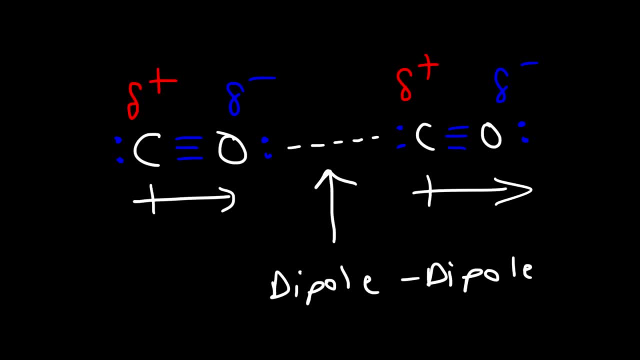 And so those two molecules are attracted to each other. As you know, opposites attract, So they feel a force that will pull them together. Now, hydrogen bonding is a special type of dipole-dipole interaction. It occurs when hydrogen is attached to one of these three elements: nitrogen, oxygen or 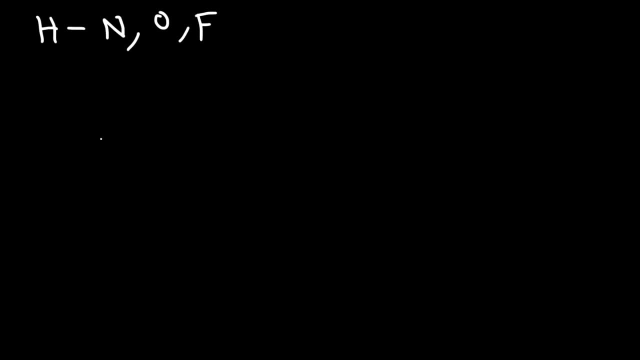 fluorine. So let's use water as an example. So the oxygen of water bears a partial negative charge and the hydrogen bears a partial positive charge, And so the oxygen of one water molecule is attracted to the hydrogen of another. And so these hydrogen bonds, or these special type of dipole-dipole, 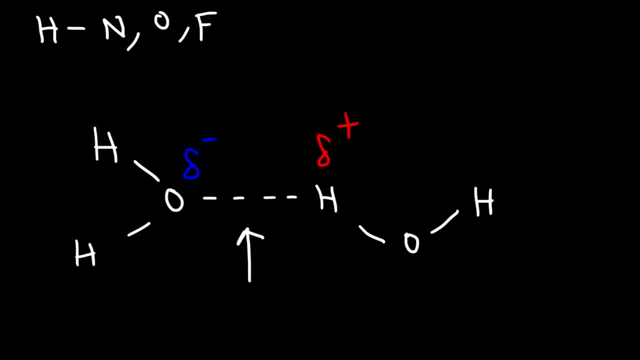 interactions. they keep the water molecules held together, And so this is an H bond. It's between two separate water molecules, as opposed to within a water molecule. Now, whenever you have hydrogen bonding, what it does to a molecule is it increases the boiling point. 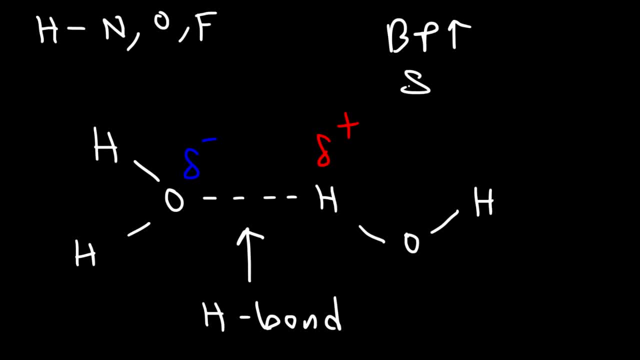 of the molecule And also it increases the water solubility of a molecule. For example, ammonia has hydrogen bonds in it And so ammonia is polar and it's going to be highly soluble in water. Methanol has hydrogen bonds in it. You can see the OH bond And, as a result, it has a 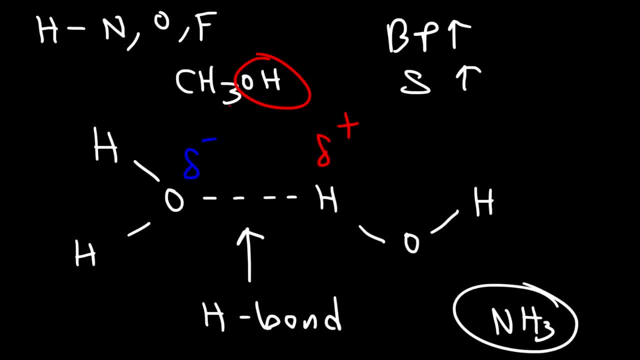 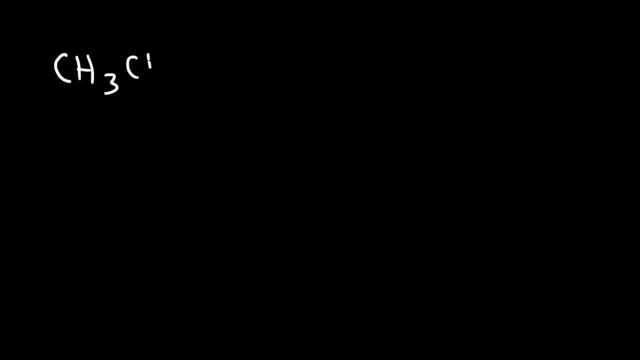 relatively higher boiling point compared to other molecules that do not have hydrogen bonds, And also the solubility of methanol in water. It is very high. Methanol mixes completely with water. Now let's compare ethanol and dimethyl ether. Which of these two molecules has a higher 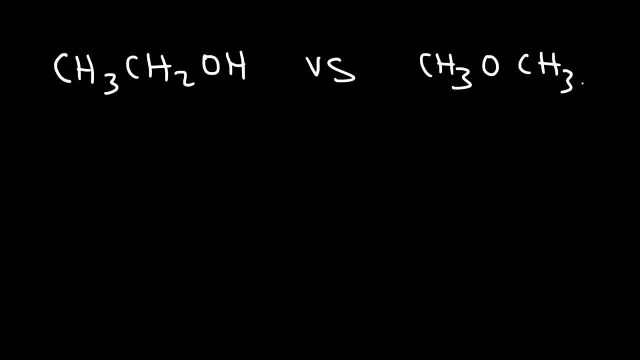 boiling point And which one has a higher solubility in water. Ethanol, we can see it has hydrogen bonds And so it's highly polar. Dimethyl ether is polar as well because of the oxygen and the fact that it has a bent shape, So it has a 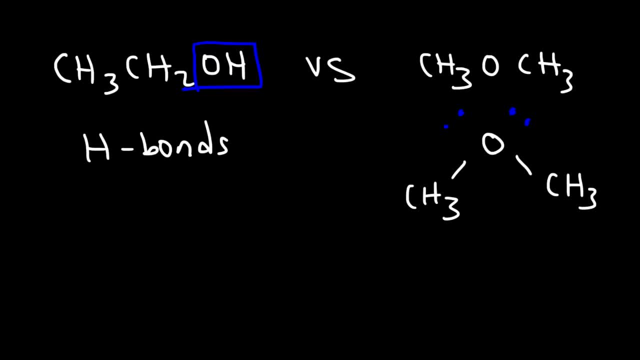 similar molecular geometry to that of water. However, notice that hydrogen is not directly attached to oxygen And so it doesn't have any hydrogen bonds. Therefore, because hydrogen bonds have more intermolecular forces, or rather stronger intermolecular forces, than regular dipole-dipole interactions, 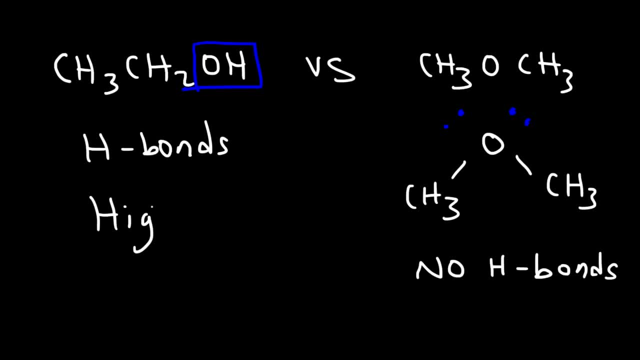 Ethanol is gonna have a higher boiling point And, as a result, it will also have a higher solubility in water. due to the H bonds, The boiling point of ethanol is about 78 degrees Celsius, And for dimethyl ether it's negative. 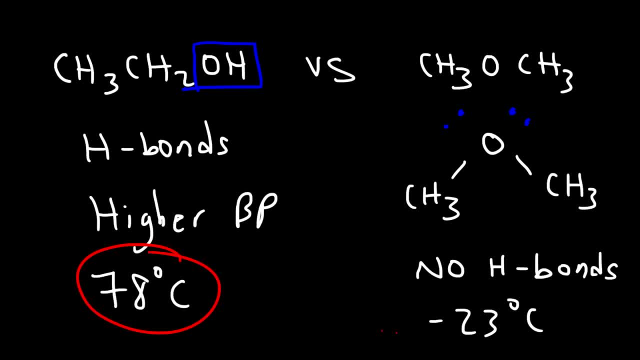 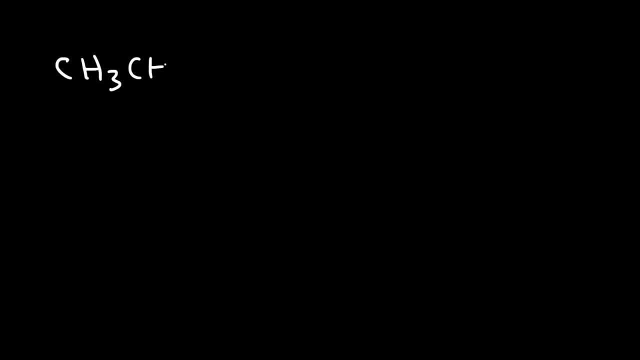 23 Celsius. So you can see that this is a lot higher than that number, And so hydrogen bonds will greatly increase the boiling point and the solubility in water- water of a molecule. Now, what if we compare ethanol with 1-butanol? Which one 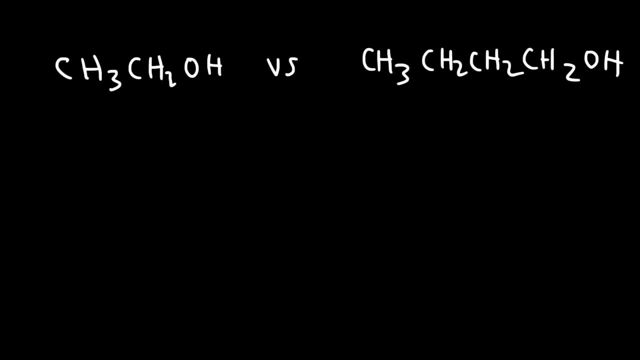 has a higher boiling point and which one has a greater solubility in water. Now, both of these molecules, they contain the hydrogen bonds. However, notice that the size of the hydrocarbon chain is not the same For butanol: there's more atoms. 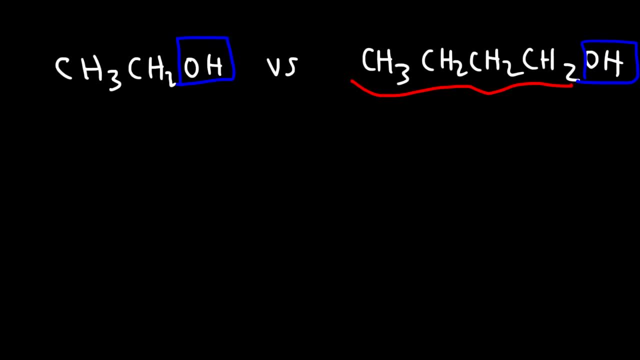 in that molecule and as a result, in addition to hydrogen bonds, it's going to have more London dispersion forces. As a result it's going to have a higher boiling point. So molecules with a large number of carbon atoms tend to have a. 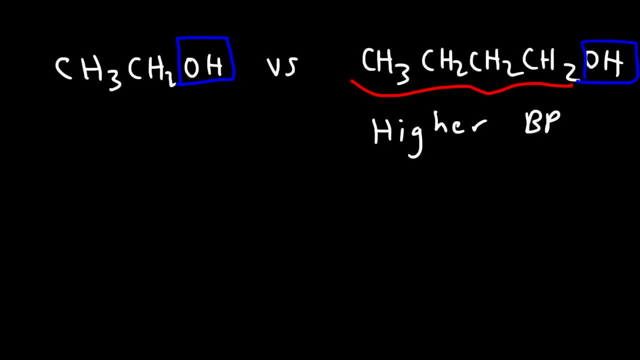 higher boiling point than molecules with only a small number of carbon atoms, Assuming everything else is the same. In this case, they both have the same OH functional group. Now, what about water solubility? Which one is more soluble in water? Now, you need to know that the OH bond is polar, but the CH bond is 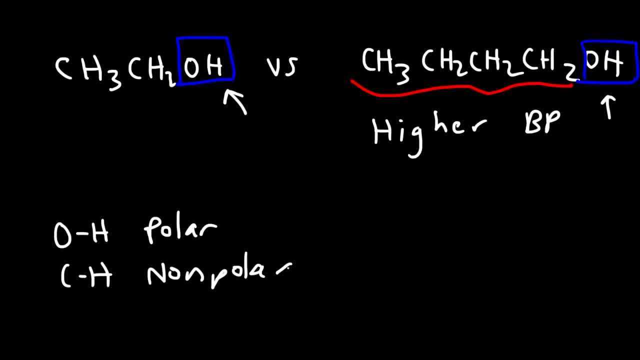 nonpolar, And water is a polar molecule like dissolves, like. So molecules with the OH group will be highly soluble in water, whereas those with a CH group will not be soluble in water. Now, ethanol is soluble in water And 1 butanol 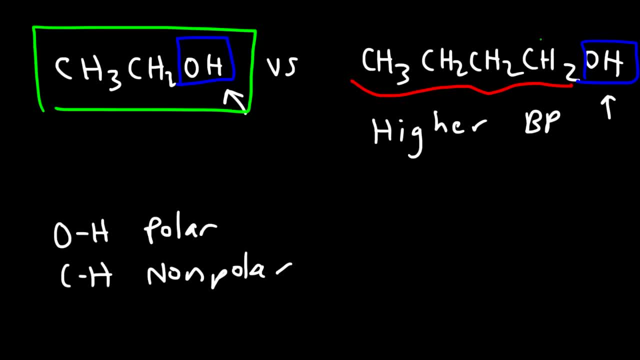 is still soluble in water. However, because of this nonpolar chain, the solubility will be less than that of ethanol. So ethanol is going to have a greater solubility in water because the nonpolar region is smaller than this. 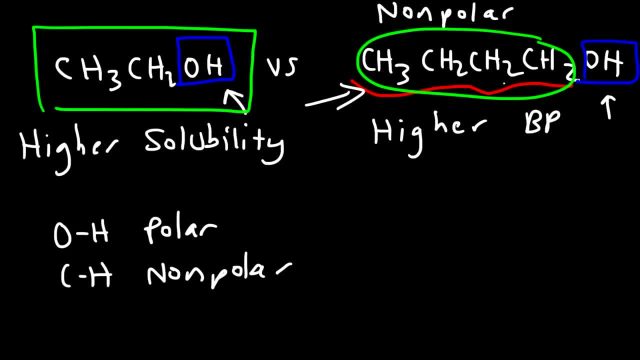 bulky nonpolar region. In fact, the solubility of butanol: it's small in water. You can dissolve some of it, but not much. Another example is 1-octanol, where we have a total of 8 carbon atoms. Now this molecule still has. 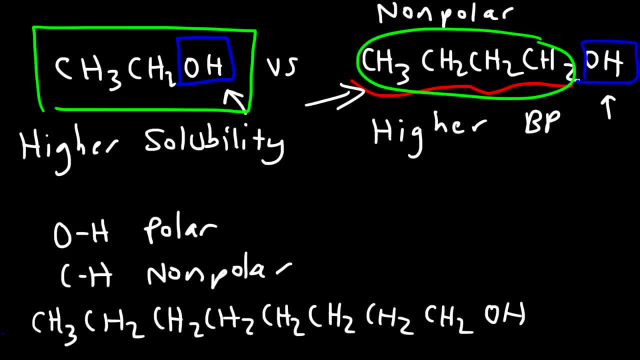 hydrogen bonds. However, because it has such a huge, bulky nonpolar region, it's not soluble in water. In fact, it mixes with other nonpolar molecules like oil and things like that, but it doesn't mix in water Because the OH part is soluble in water but the CH 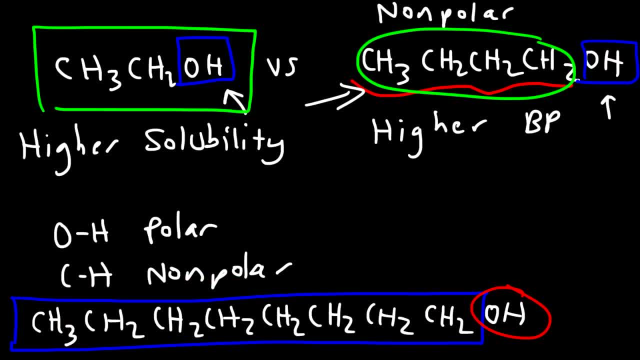 part is not. The CH bonds are nonpolar, so they don't want to mix with water, And so whenever you have small chain alcohols like ethanol or even methanol, these are highly soluble in water. But when you start adding a lot of CH groups or CH2 groups, you're going to notice that the soluble is going to decrease but the boiling point will go up. So 1-octanol has the highest boiling point of these three molecules, But methanol has the highest solubility because it has the least number of nonpolar bonds.